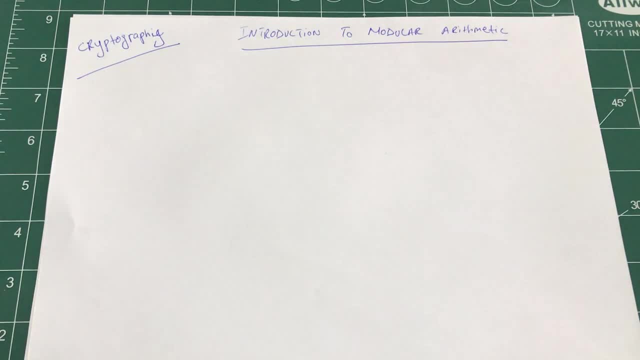 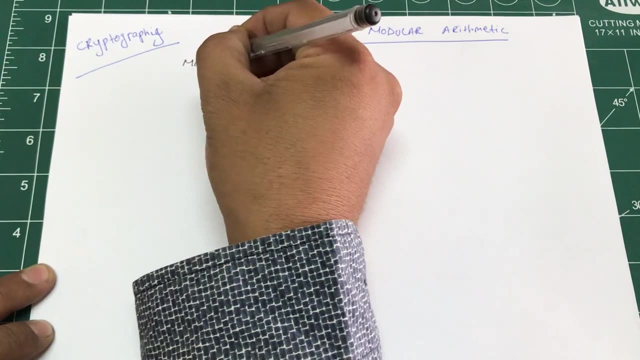 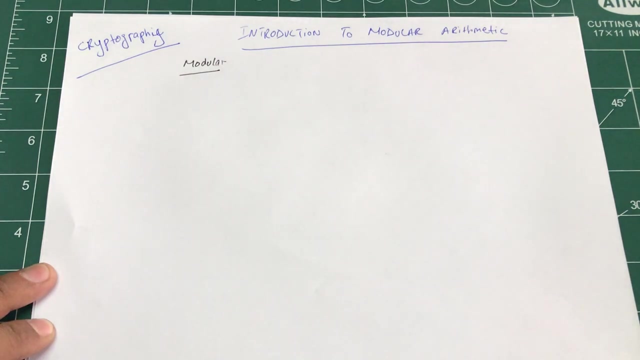 this and let's start by introducing some basic things that we need to know Basically in Modular Arithmetic. we're looking for modular properties- Modular properties we use in cryptography and other things like that- and we're gonna look at some of the operators. 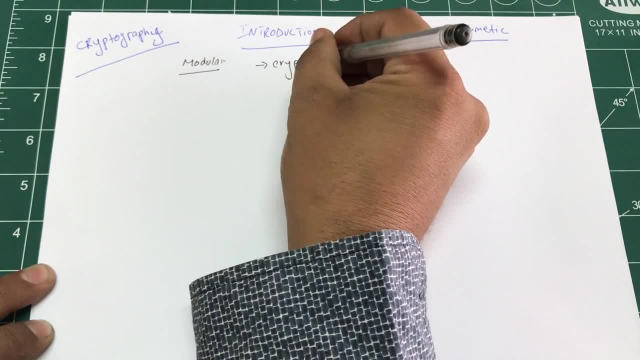 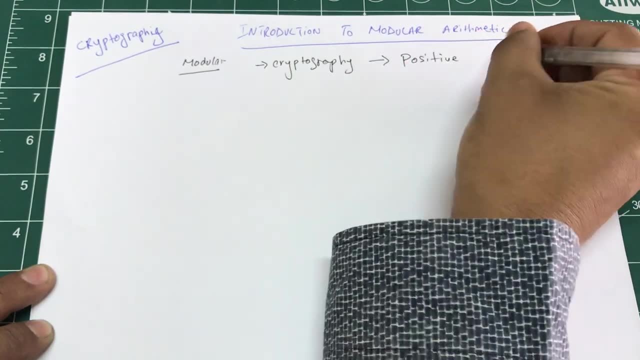 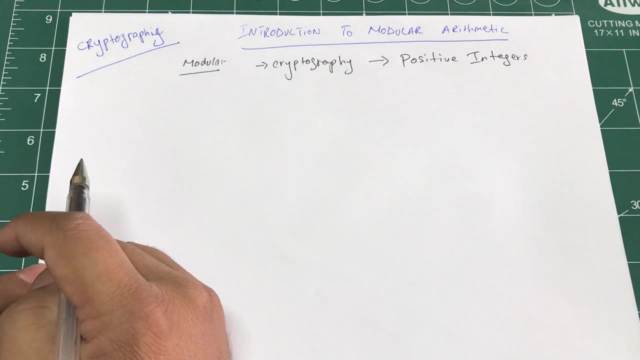 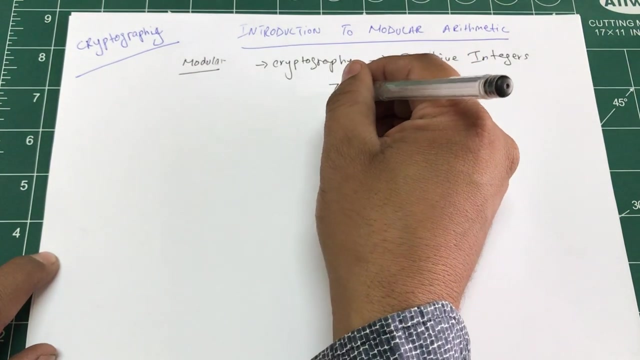 So always remember that cryptography is done usually on positive integers, So we're only focusing on positive integers. This is what cryptography focuses on: on positive integers, On positive integers. and specifically, the domain that we're going to look at today is the domain that we have for z, which is for integers, is going to be n. that is going. 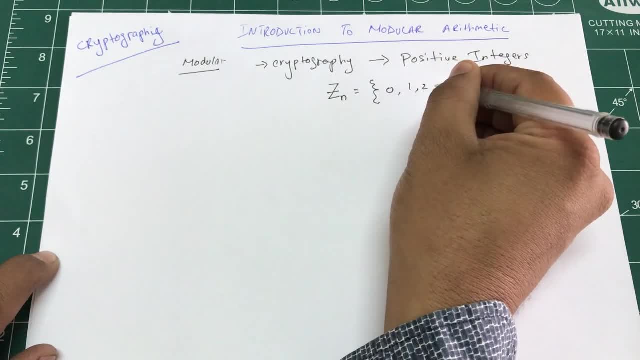 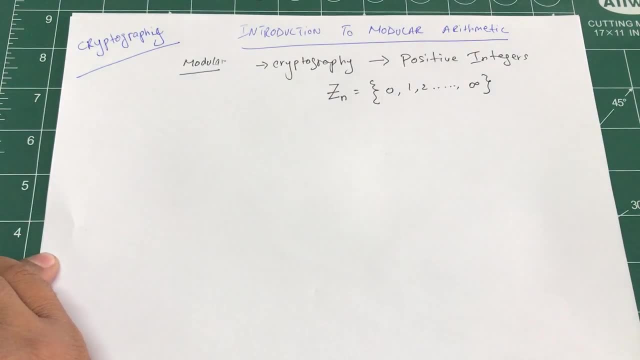 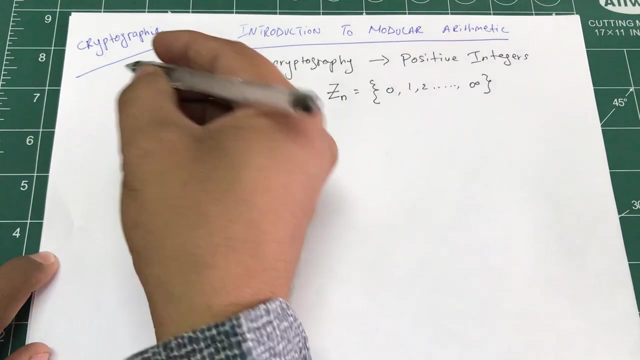 to be from zero, one, two, all the way up to positive infinity. These are the numbers that I'm interested in. So the first operation that I'm focusing on. we're just gonna go to an example. So what do we have? What type of mathematical operations we have? So mathematical? 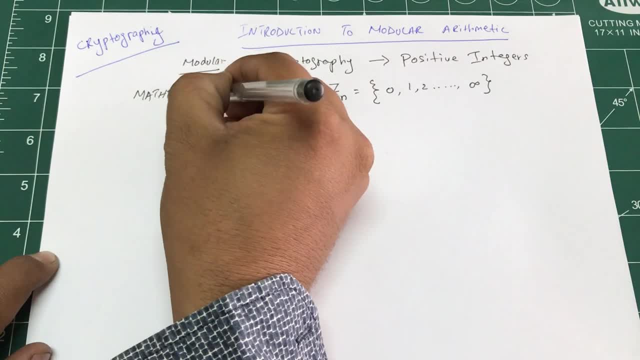 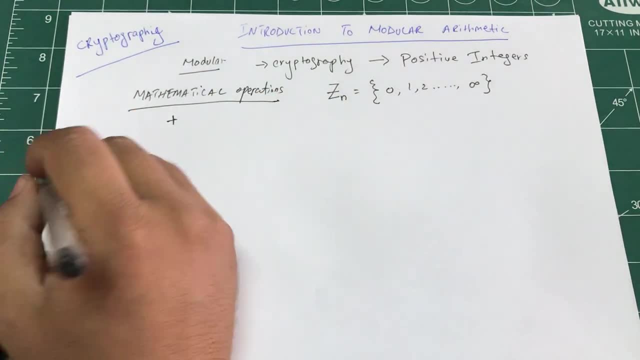 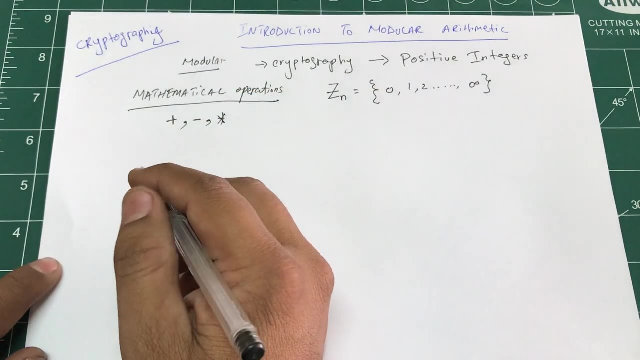 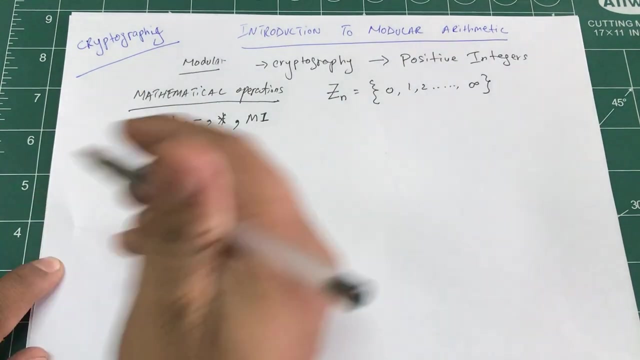 operations that we have in cryptography. We have plus addition, we have subtraction, we have multiplication and we have something called instead of division, we have something called multiplicative inverses. Let's just call it mi for multiplicative inverses. We're gonna learn that in the next tutorial. how? 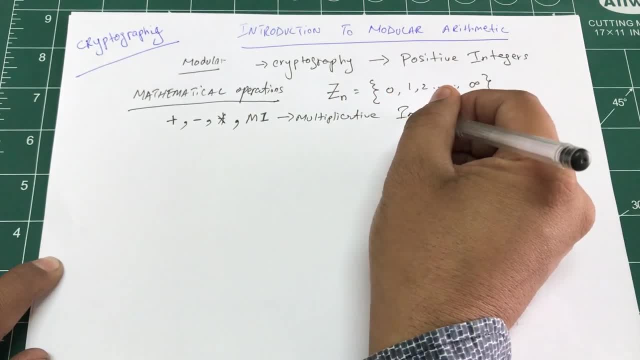 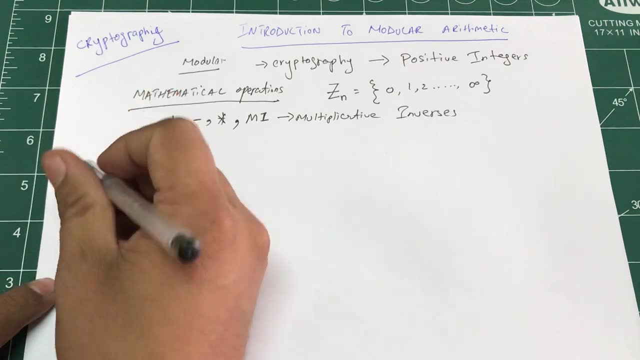 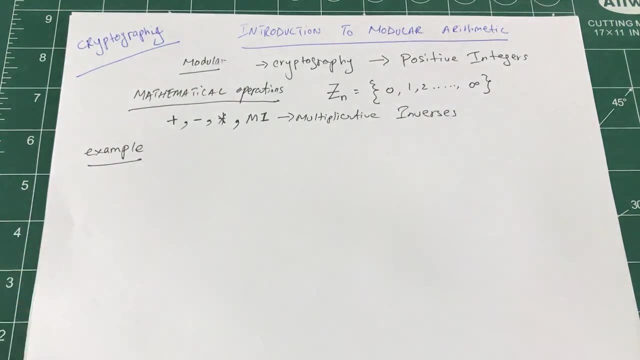 to find multiplicative inverses of things. Multiplicative inverses, That's what we're focusing on. So let's look at, let's do an example. So, instead of focusing and wasting your time, let's do an example. Let's say I have given a problem, which is something. 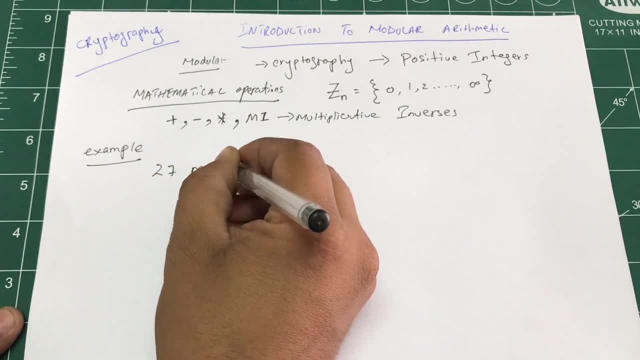 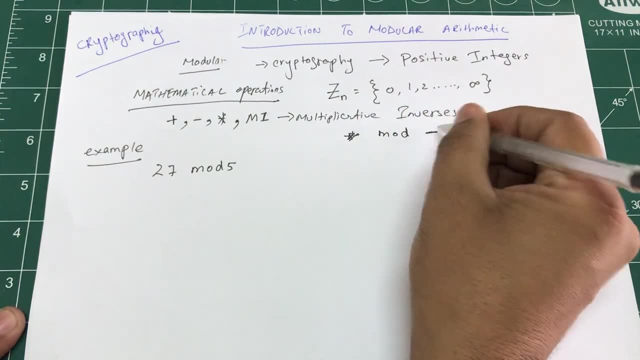 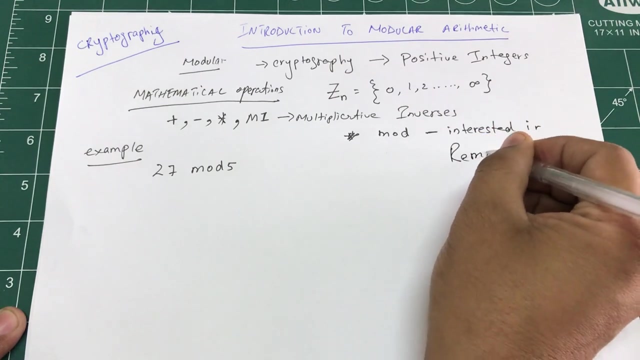 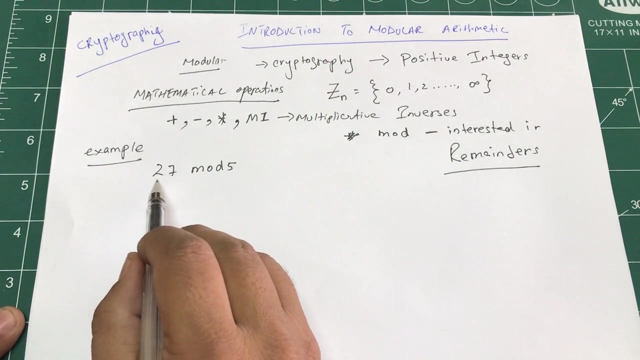 like this: 27 mod five. Always remember that in mod, we are interested in remainders. We only care about remainders. That's all we care about. We only care about remainders. So what we're doing is this: We're gonna divide 27.. We're gonna take a mod with five, So in 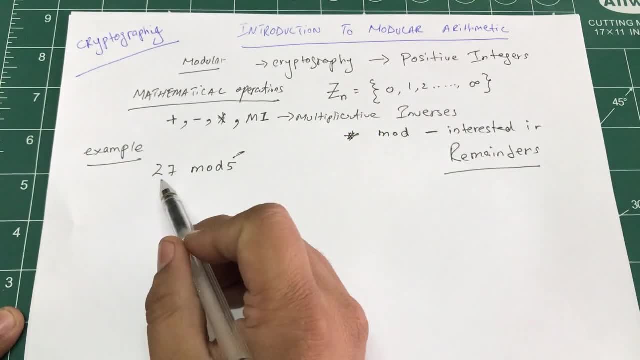 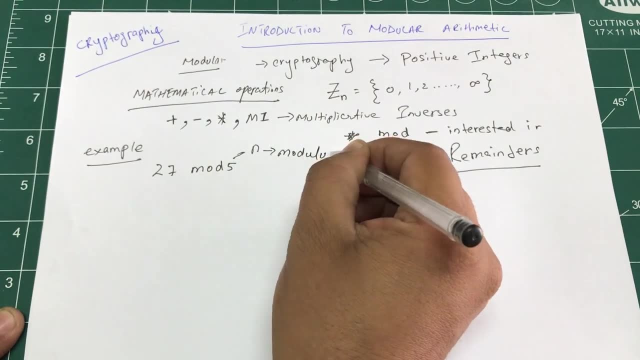 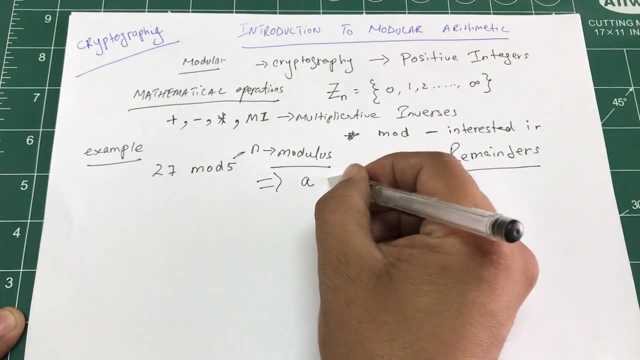 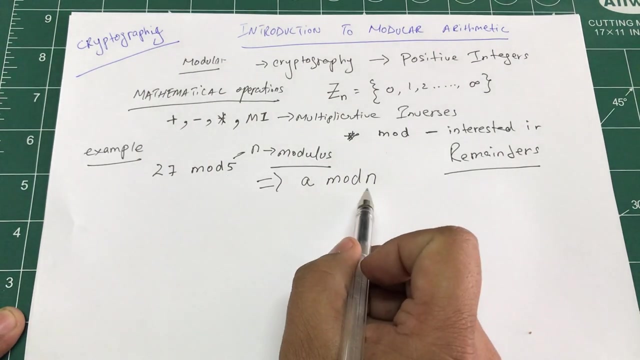 cryptography. we're gonna call this guy who, which we're dividing by n, which is known as your modulus. All right, So this is in general form. This. this thing looks like in general form. This looks like I mod n, So this number is going to be your modulus. In generic form, this is known as: 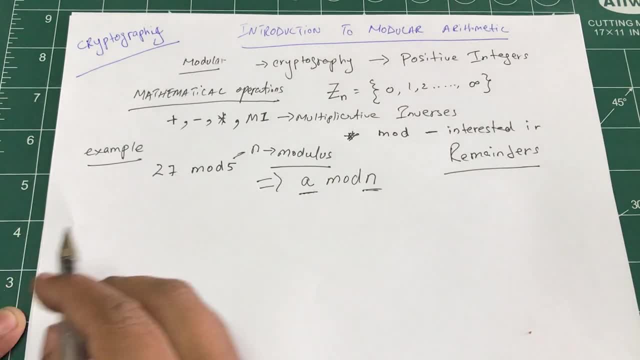 n, And this is the number that I'm dividing. So, basically, what you're doing is this: You're taking 27.. You're dividing 27 by five. So 25 times five would gives me 25.. And what is the remainder that I get? 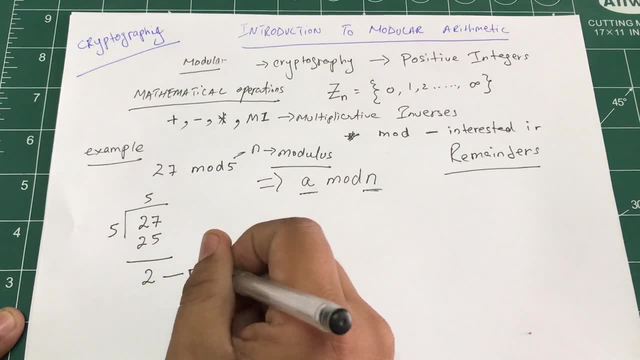 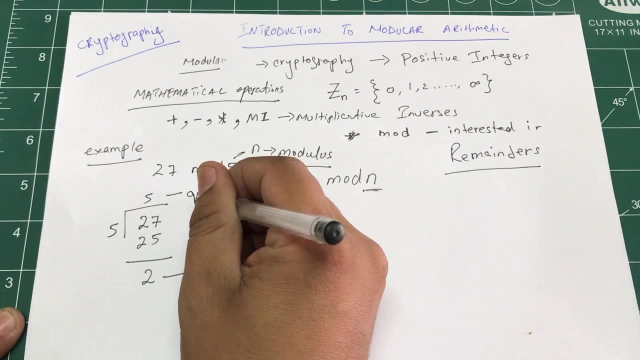 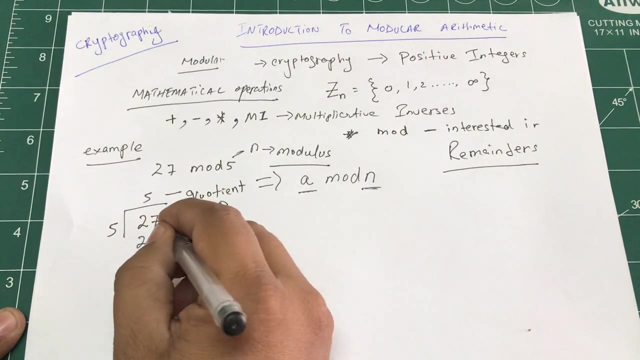 Is two. So this is going to be your remainder. All right, This is going to be your quotient, which is a quotient or Q, And this is going to be that number, which is a, and this is going to be your number, which is going to be n. All right, That's all. That's all I. 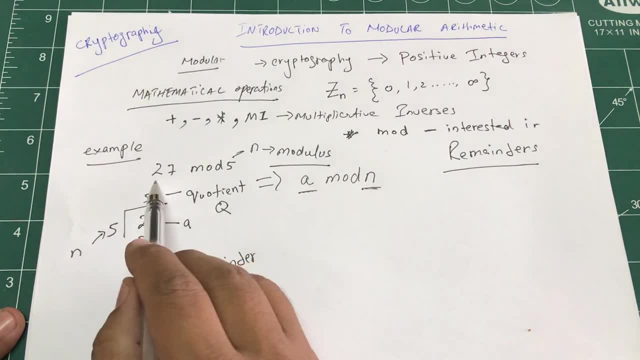 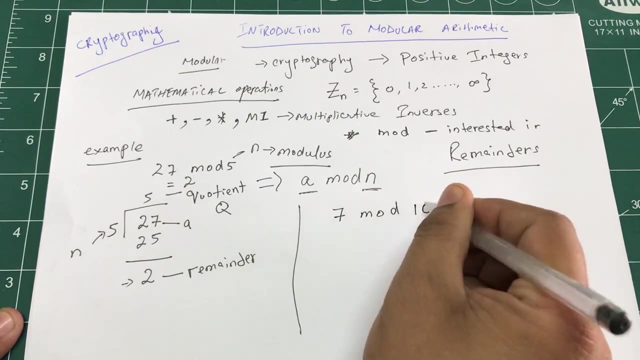 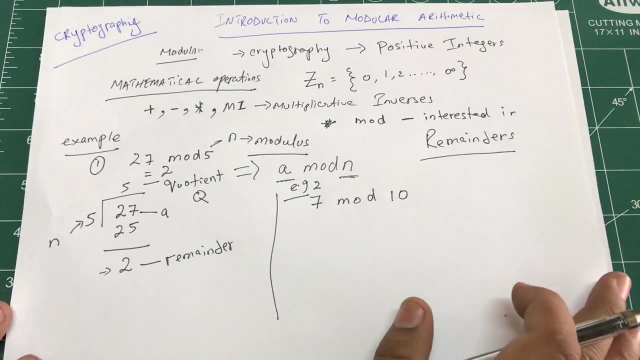 need to do in order to do modulo arithmetic. So 27 mod five. The answer of this guy is two. Okay, let's do one more example. Let's say I have something like this: Seven mod ten. So example number one, Example two: What is seven mod two? So always remember, 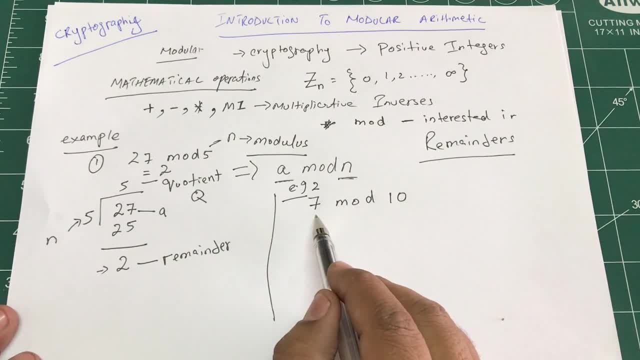 that when your modulus is bigger and the number is smaller, you get the same number back. That's all you need to remember when you have your modulus. So the rule is that you get the same number back when you have your modulus. So the rule 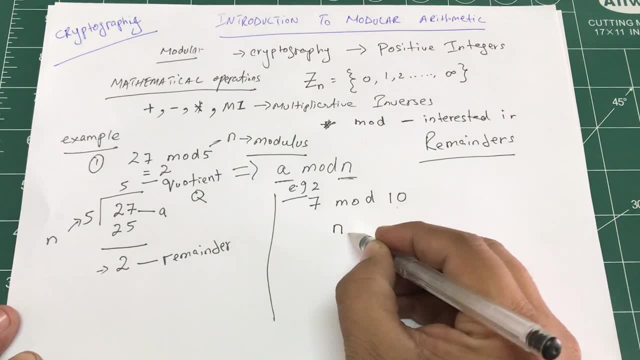 is that you get the same number back when you have your modulus. So the rule is that you get the same number back when you have your modulus. So the rule is this: When you have your modulus, n is greater than greater than not equal. 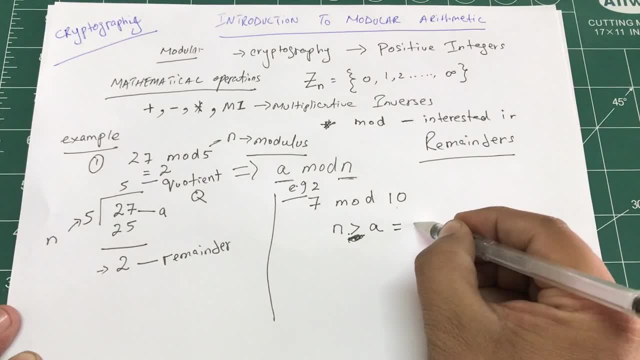 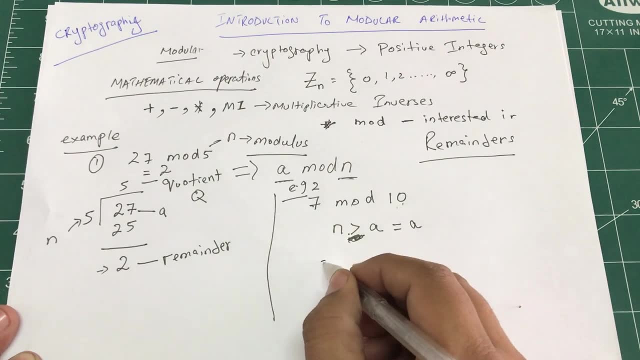 to greater than a, you get the same number. Answer is a. All right, So seven mod ten, you'll get the same number back. So the answer for this guy is going to be seven. I hope you got this. So when you have n, which is a modulus, which is going to be greater than, 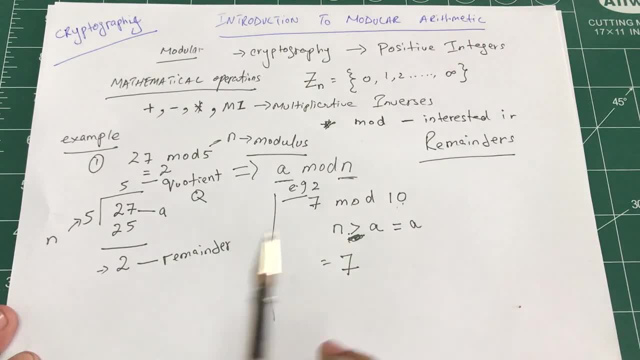 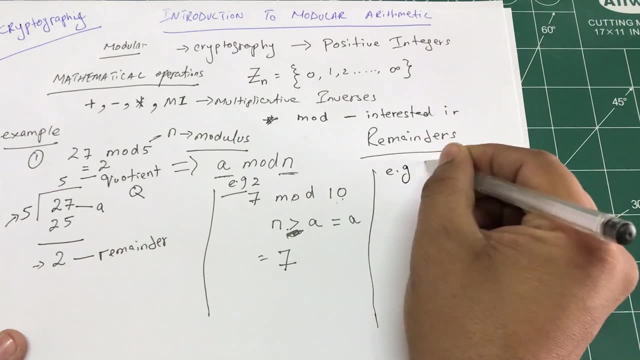 a this number, you'll get the same number back. that's it. okay. let's do one more example. let's do example three. example three: let's say i have a negative number. so let's do example three like this: let's say i have a negative number, negative. 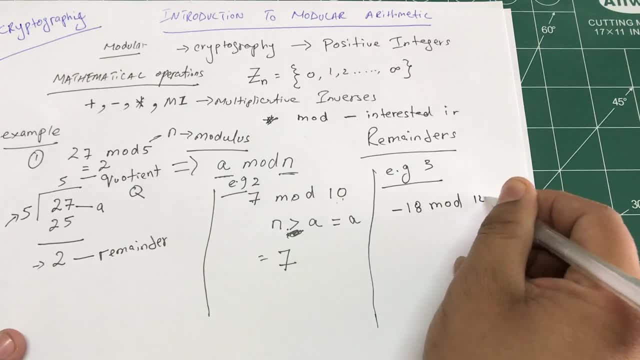 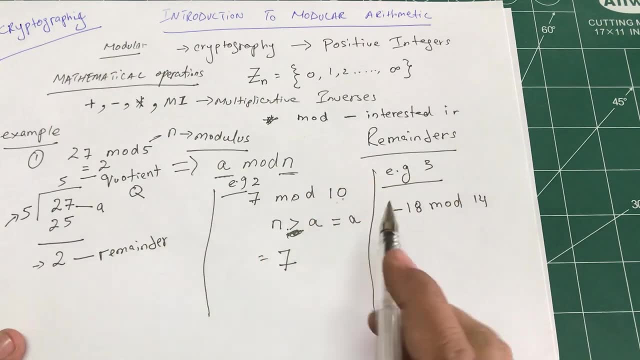 18 mod 14, all right. so how am i going to solve this? so i know this guy is bigger, so we're just going to ignore the negative and we're going to treat this as a normal mod problem. so we're going to divide 18 by 14. so what is it? 14 times 1 is 14. the remainder is 4. so this is my remainder. 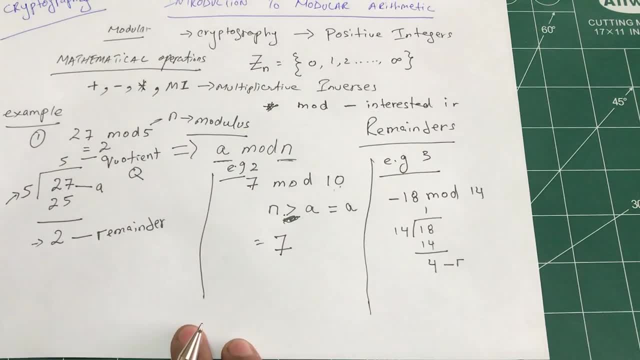 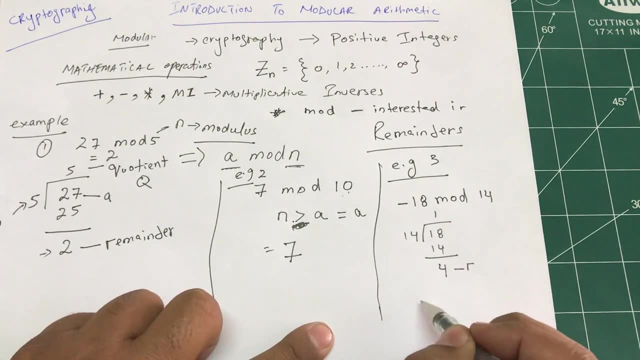 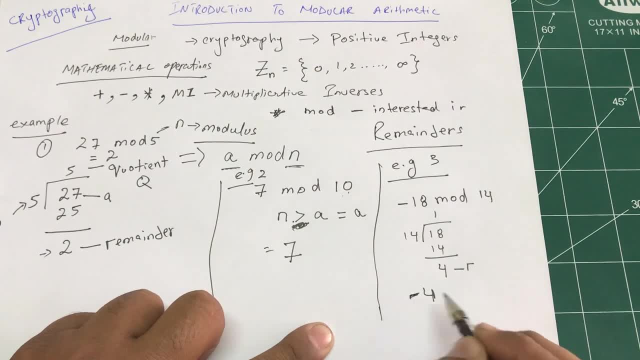 bring this negative out as well, and then i'm going to add my modulus in this number. so i'm going to add my modulus in this number. so what do i get? 14 minus 4, i'll get 10. so the answer for negative 10 mod 14 is going to be 10. i hope you got that. so what about if negative 10 mod 14? 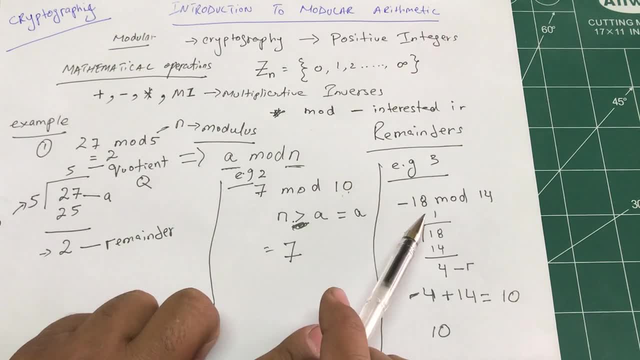 all right, how am i going to solve this? i'm going to treat this as a normal mod problem, all right? uh, since i i'm only interested in cryptography and we're only interested in positive integers, that's all i care about. so i'm going to do 18, mod 14. i'll get a remainder of 4. 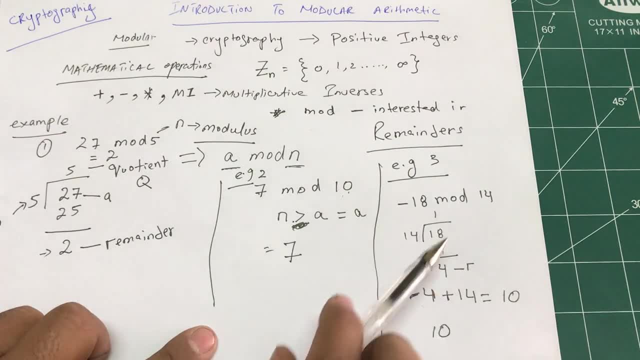 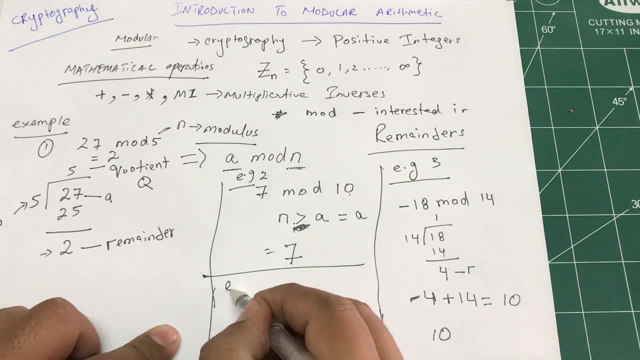 then i'll write my 4, i'll bring that negative out and i'm going to add my modulus in it, whatever the answer i will get. that is going to be my answer. all right, let's do example one more example, example number four. let's say i get something like this negative 7 mod. 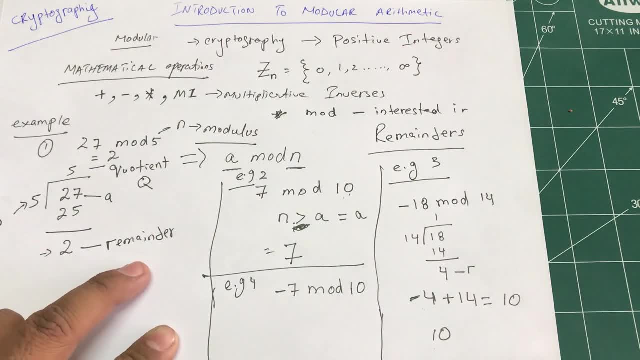 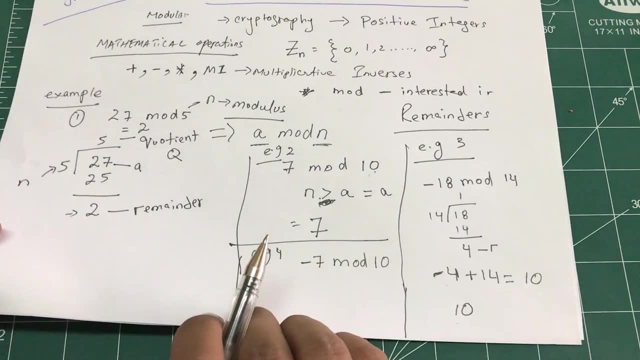 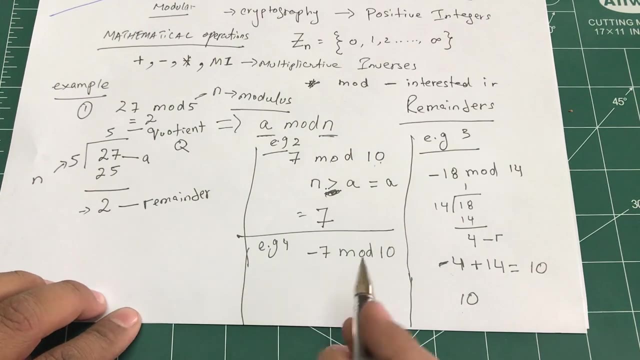 10. all right, i'm going to treat exactly the same way, just like i have done it previously in the example number two: any number. so i'm going to ignore the negative. if my modulus is bigger than my number, i'm going to get the same number back. so i'll get what 7 and i'm going to bring. 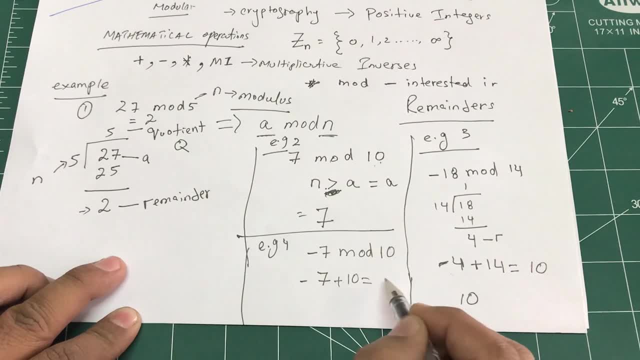 that negative out and i'm going to add my modulus, so my answer would be 3, so this is how you solve it. that's all you need to know. uh, regarding, uh- cryptography, modular arithmetic, uh, that that we would do in our cryptography series. one thing that i want to make sure is this one: 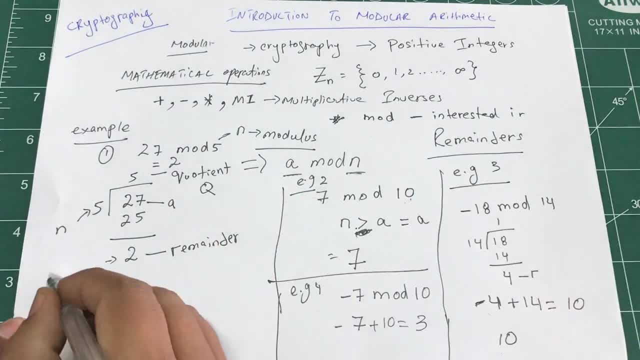 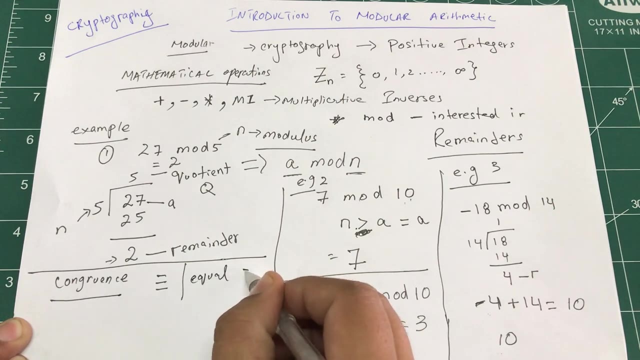 operation that i want to include is this, which is going to be a congruence operation. the symbol for congruence is actually three bars, like this, and for equal, for equal, you get two. what congruence is? what congruence is that many number will map onto a particular value. 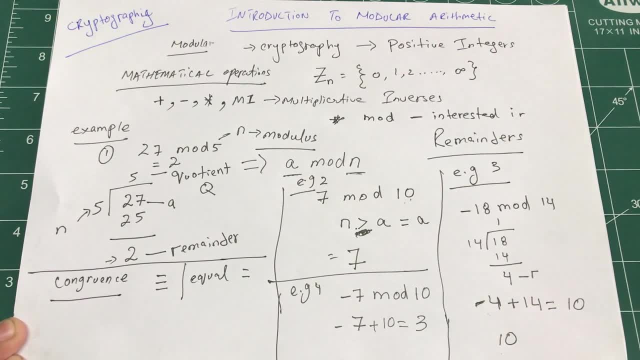 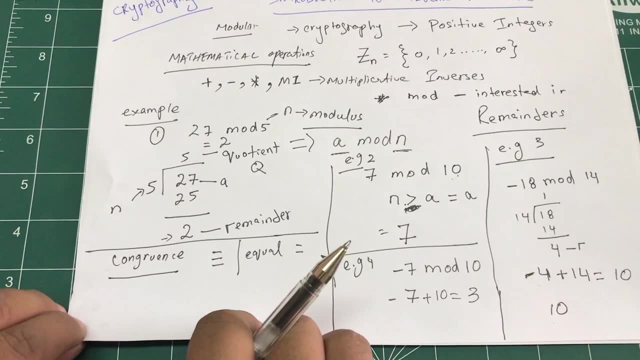 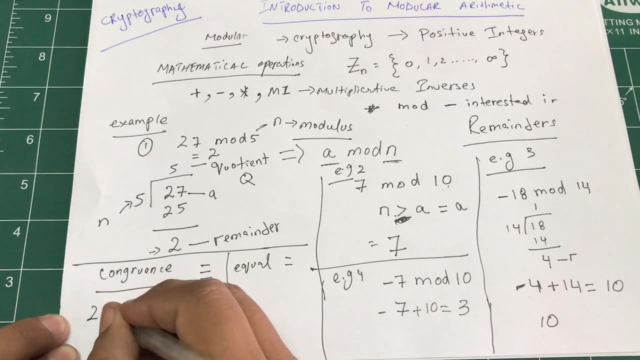 all right, this is what congruence is. many number will map into a single value. so let's, let's look at an example. this is also one of the most common operation that we like to use in cryptography as well, which is okay. so i have a number like this: uh, two congruence, 12 mod. 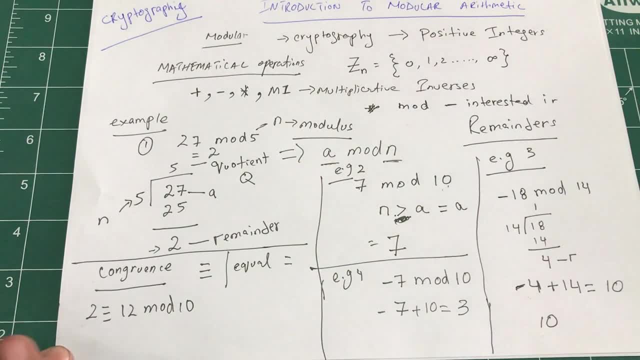 10, okay. so what is it that i'm doing? ignore, ignore this two for right now, and let's look at this problem. what is 12 mod 10? 12 mod 10 would give me two, okay, but since i have a congruence operator, what congruence congruence operator does is just not 12 mod 10 and will only give. 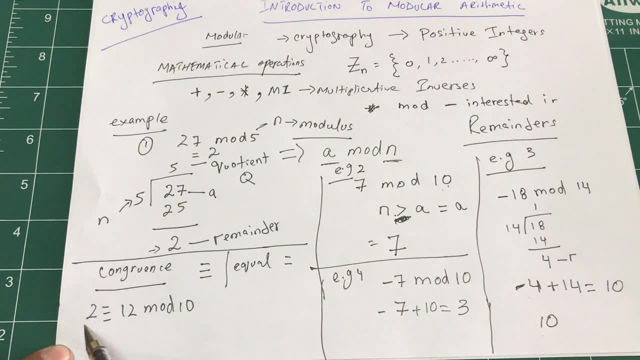 you two. what about 22 mod 10? you will also get two. what about 32 mod 10? you will also get two. so many values in this modulus domain would give you this number. on the other hand, equal means: this value is equal to this. okay, this value is equal to this, while in congruence, many different. 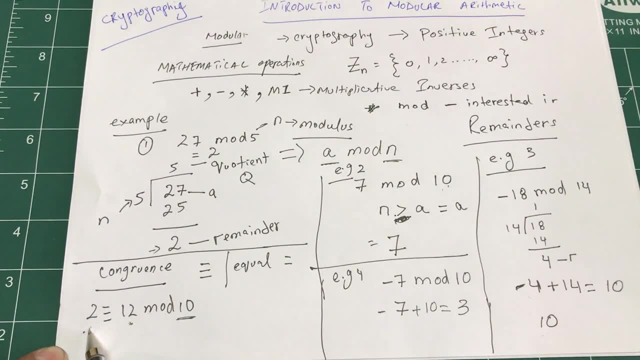 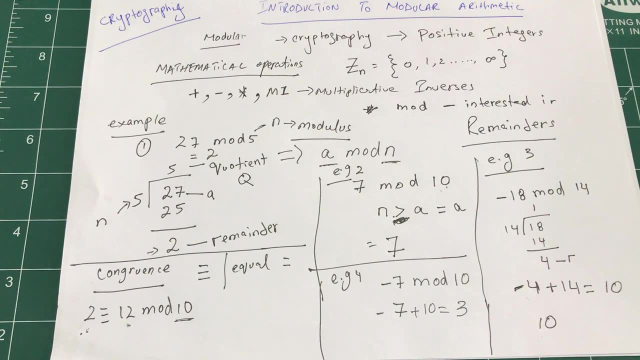 value of your number would map into the same value. so this is one of the operation that we like to use in in in cryptography, so don't forget to subscribe to the channel and i hope you like the video.